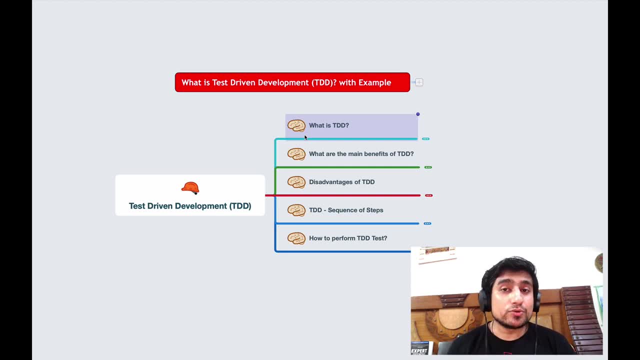 Hey guys, welcome to testing academy. My name is Pramod and welcome to the series of 30 days of automation and testing. In this video, we are going to talk about the what is test driven development with an example. We are going to talk about what the major benefits, disadvantages, sequence and steps, and how to perform the TDD. I'm going to show you one practical example And, trust me, guys, this is one of the topic which is important for your interviews, right? If you are anyone who is preparing for interviews and they are going to ask about TDD, right? So I'm excited to show you how to perform the TDD. 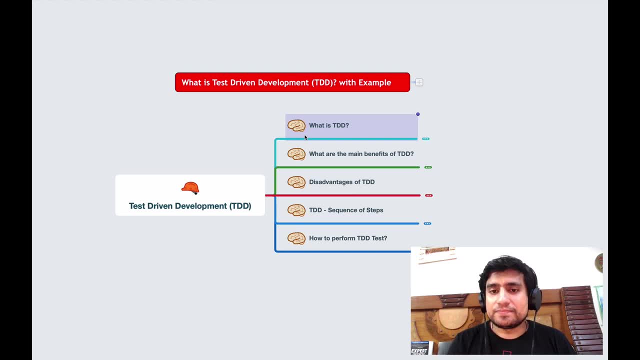 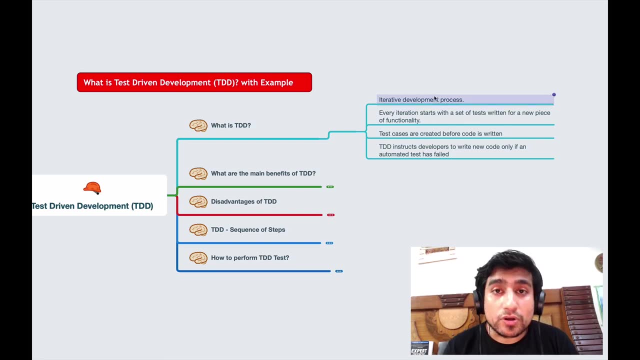 I'm excited to show all the things, All right, so let's get started. All right, All right guys. So let's start with a quick example. What is TDD? right? TDD is basically an iterative development process, right? So what we do in here is that in TDD, is that every iteration starts with a set of tests returned for a new piece of functionality. So, basically, in a very simple manner, if I say, is that first you will prepare a series of test cases, right, You are not preparing the functionality of it. Let's take an example. 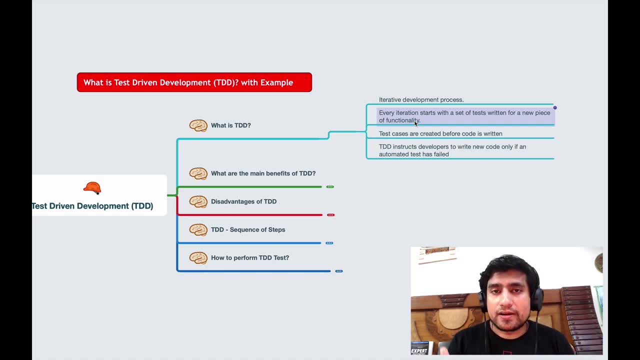 You have a username that you want to validate, right? So this username should not contain spaces, should not contain any special characters, right? So these are test cases. right, It should be a valid username. Basically, it contains only the ABCD, and all right, And it should not contain special characters. It should not contain, at the rate, hash or something like this, right? So first thing is that you will prepare certain test cases. You will fail them. 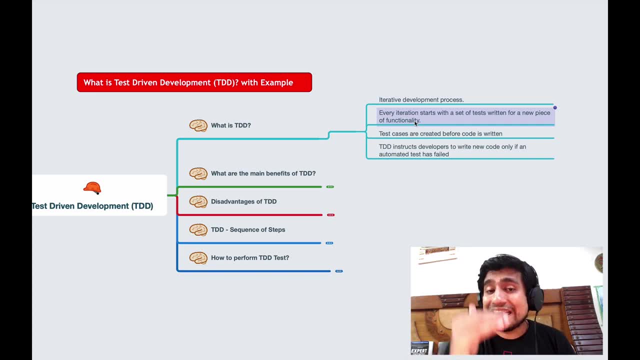 And after that you will write the code according to it And in the end what you will have is that you will have a test which is basically driving your development effort And in the end you will have a particular function coded which can handle all the test cases right. It is one of the best way to do development process right. So test cases are created before the code is written, And TDD basically instruct the developers to write the new code only if that automated test that we are running is basically has paid right. So 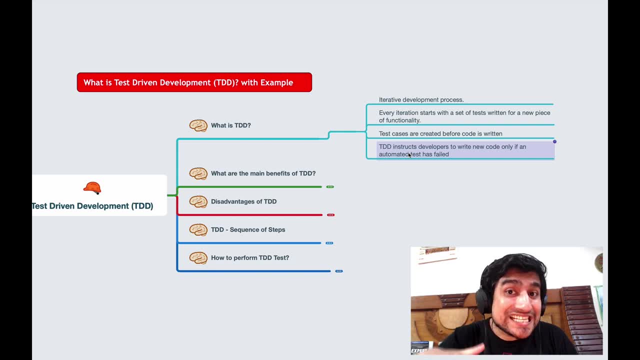 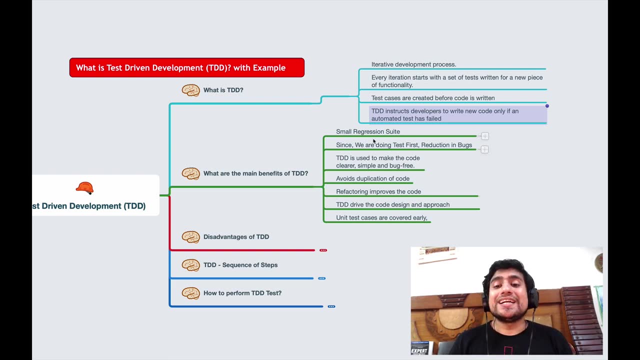 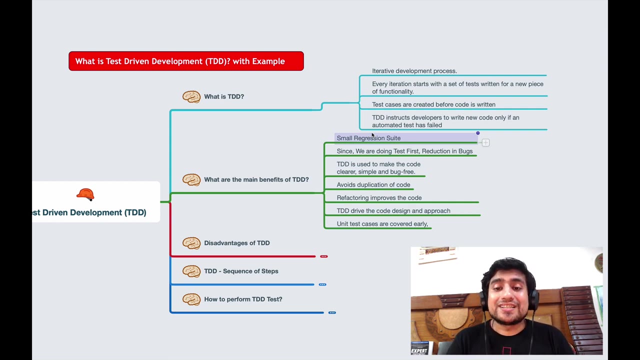 if you are not able to get it, let's see in the example, in the demo part. right Before that, let's jump into what is that main advantage of a TDD? right? So TDD, if you have taken this development process right, TDD, there will be like small regression suite, Since we are doing tests first. so there will be a reduction in bugs. right, Because your tests are basically your test. the test cases that you have created are already handled into the code. right? So there will be a reduction in bugs. 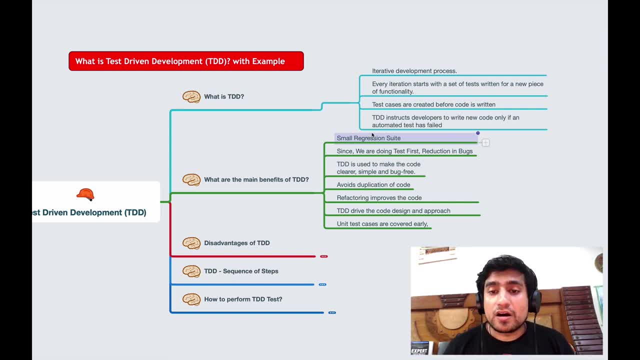 That's why TDD is so popular. TDD is used to make the code clearer, simpler, with bug free. It avoids duplication. refactoring, basically refactoring of code is improved because we have mapped the test cases with the functionality that we have written. TDD drive the code design and approach. Unit test case are covered early right Because most of the cases that we have already returned, so unit test cases, are covered in the early phase of it. So major disadvantage is that early 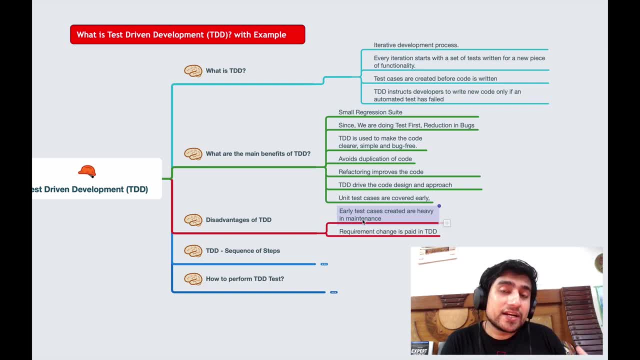 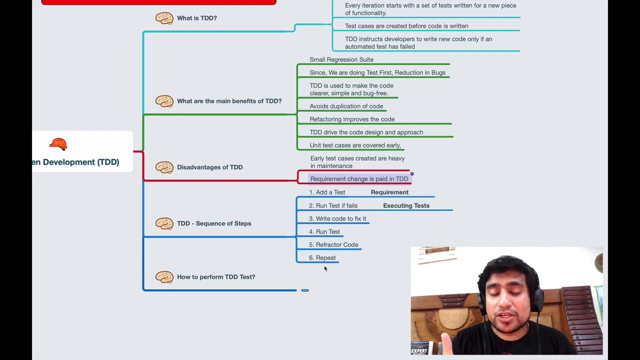 test cases are heavy in maintenance because we are already creating a test case. Suppose I have created a 50 test cases and developed a functionality. Now the test case is failing or something bad is happening, right? Maintenance cost is high in that case. If the requirement are changing, test case will change, maintenance will change, development effort will change. So that is again very disadvantage in that case, right? So how do you do? how you perform the TDD? They are like sequence of steps that you need to do First thing. first is that you will read the requirement, you will add the test cases to it And after 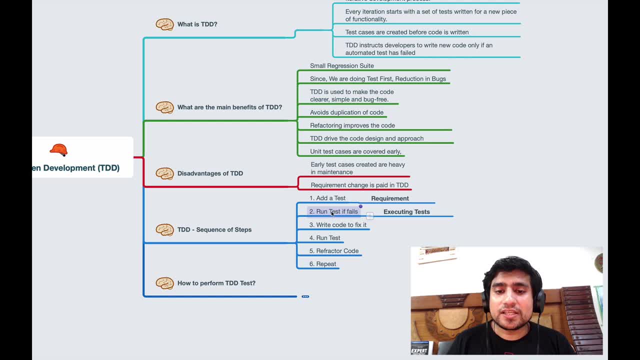 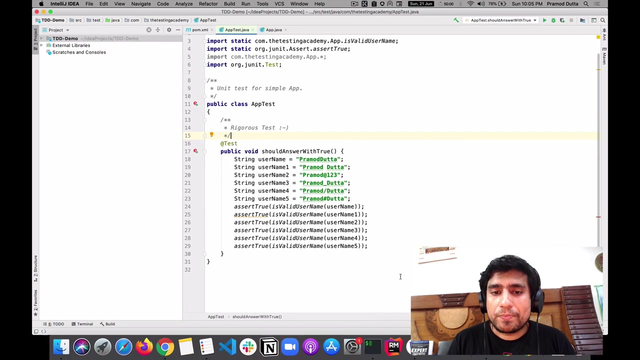 that you will run the test case and basically it will fail all those things. You will write the code to fix it And after that you will basically run the test again. If they are passed or not, you will refactor your code And again you will repeat the same process until your all test cases will pass and your functionality will be completed in that case. So how do we perform it? It's very simple: Add code, execute, write code, repeat. So this is a very simple process, right? So let me show you practically what do you mean by this. So what I have done is that let me show you. 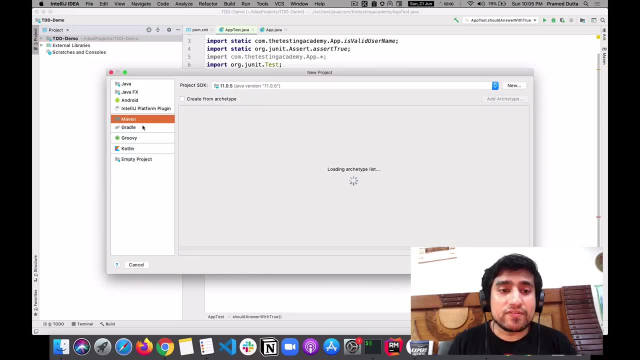 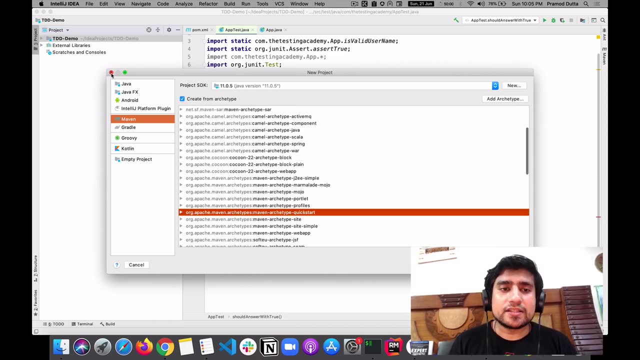 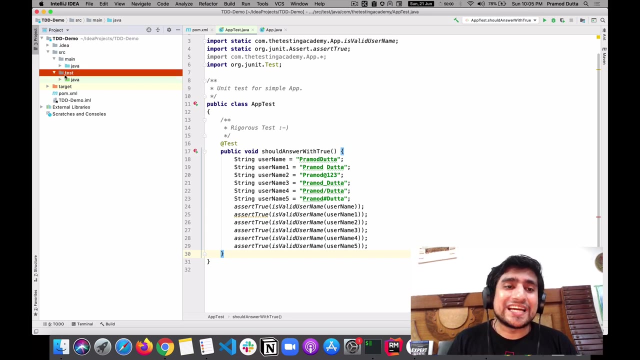 So if you click new project, let's create a new Maven project. click on Maven From archetype. I will recommend you to start with quick archetype. click next and the project will be created for you, right? So you will see two folder, which is the main folder, where you will write your development code. In the test folder, you can write your test cases, right? So, since it's a TDD, what you need to do is that you need to write the test cases first. So what I have done is that. so if you 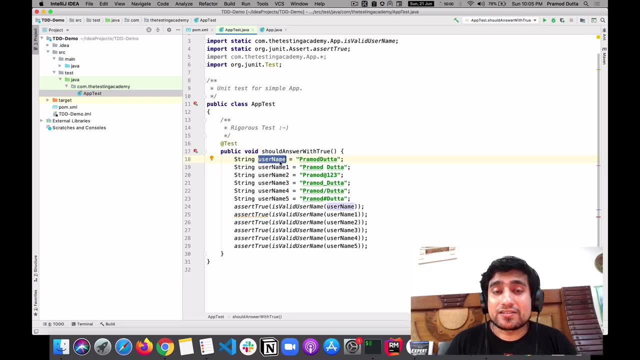 are. So what I have done is that I have created certain strings. So these are like certain test cases. So my first username will be Pramod Datta, with no you, no spaces, right? This is a very test case with space. I don't want it because this is not against the functionality, against the requirement, So this will be a failure case. I don't want. at the rate. this will again be a failure case This way. this is a negative. again, you underscore is not allowed. This is not allowed. This is not allowed. right, And what I am doing here is that I am 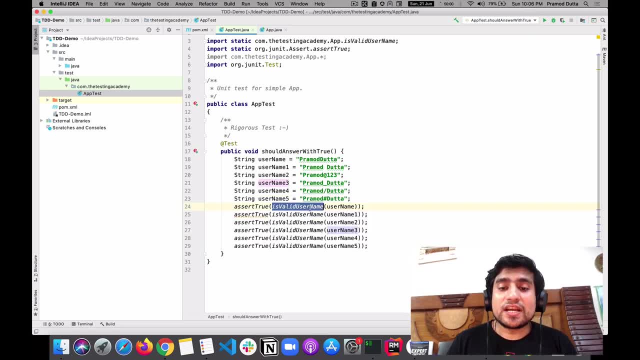 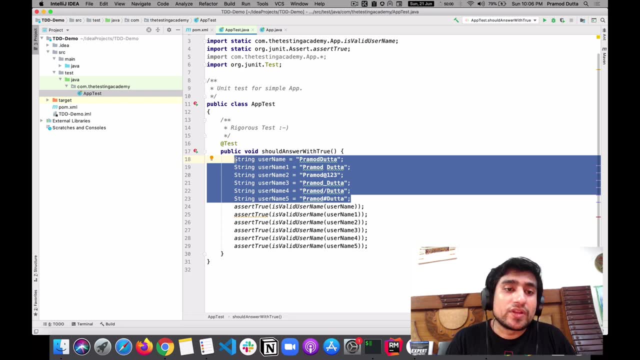 asserting the value. right? so this is the function that we need to develop, right, so we haven't developed it. this is the test case that we have written, so these are like couple of strings that we need to do, so let's jump into it, right? so before before doing it right, this is the function. 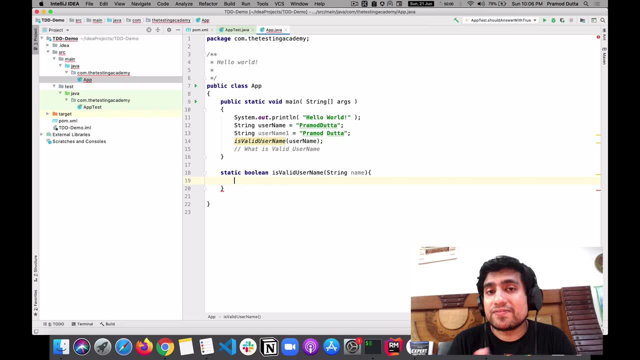 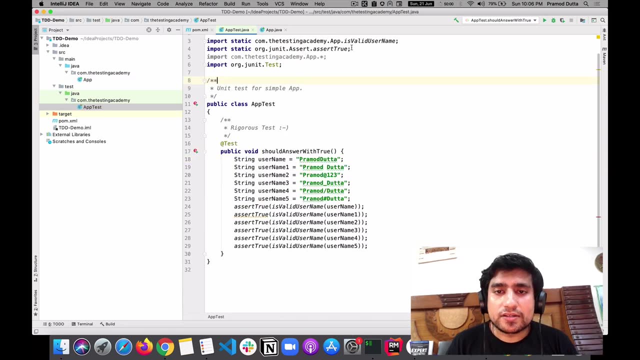 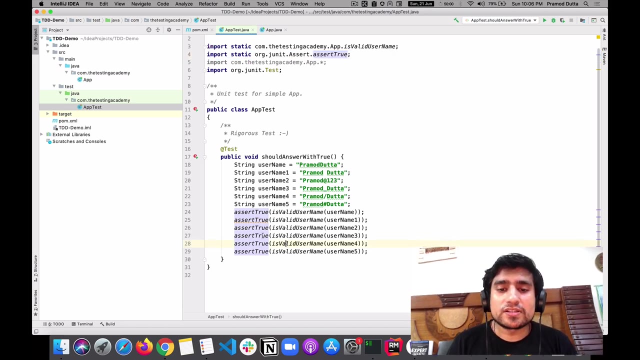 which was empty, so let's suppose this was empty first, right? so all our test cases will fail. so what i have done is that uh here, if you see i have imported it right so you can import the function here. we have imported the assert true and this function returns uh boolean value, so it will. 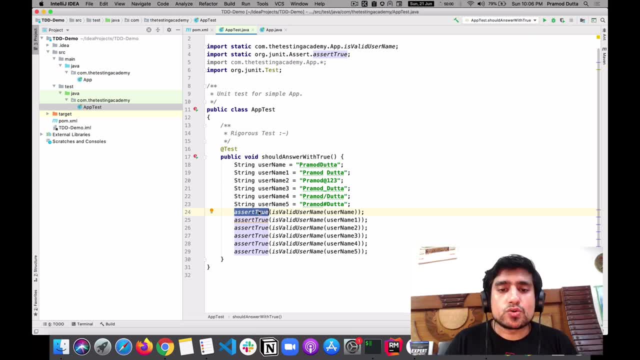 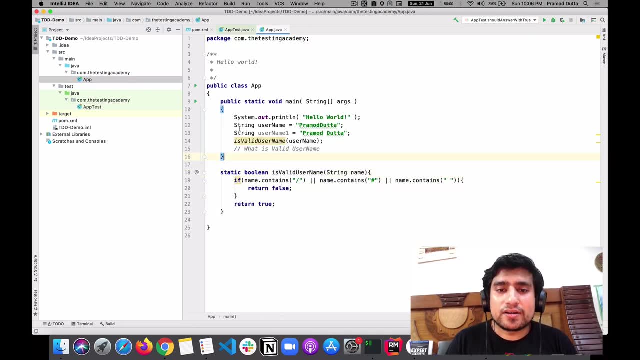 result. uh, we want to basically check for true always. so if it is failing, is it not a valid user? it will fail and again our assertion will fail right. so in tdd, what we are doing here is that uh, ignore this part. uh, we are calling the function right. so, uh, i'm using this function and 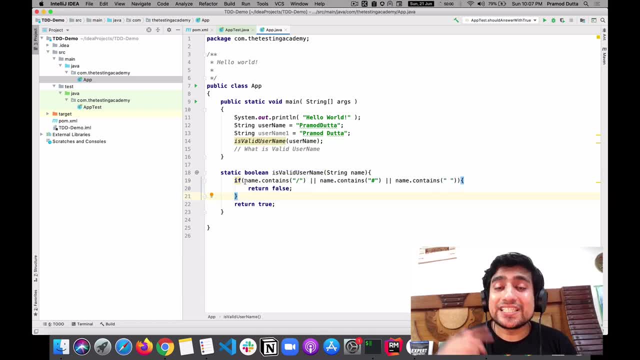 now what i'm doing is that i'm writing the conditions one by one. so the first, the first test case word it's will be a valid string right. so if it is a valid string will return true in that case. so if the name, which is the username, if it contains slash, we want to fail it because this is not a valid right. 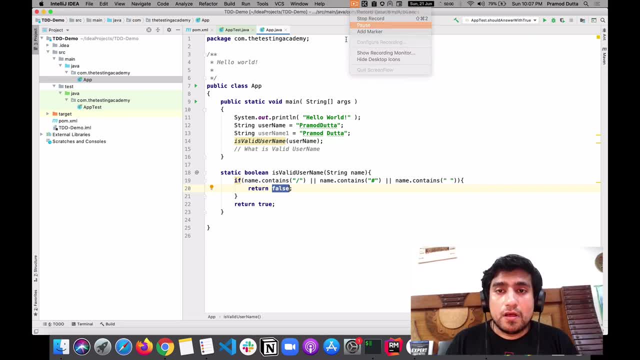 it will return false. in that case right. and similarly, if it contains hash, if contains space, will basically fail the test in that case. now your test cases. i have written the test case first and after the uh. i have written the implementation of this code right. so now i can use this code somewhere. 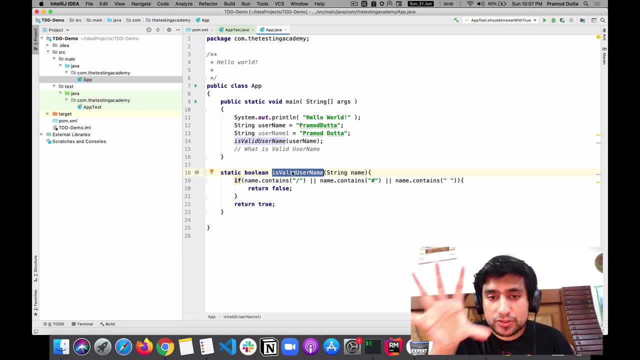 if suppose i'm developing a particular form, and all right. so here we have used a tdd approach, where we have a test cases first, and after that we have developed the functionality. so this is the. this function is now complete- assuming it is complete as of now- and what you can do is that. 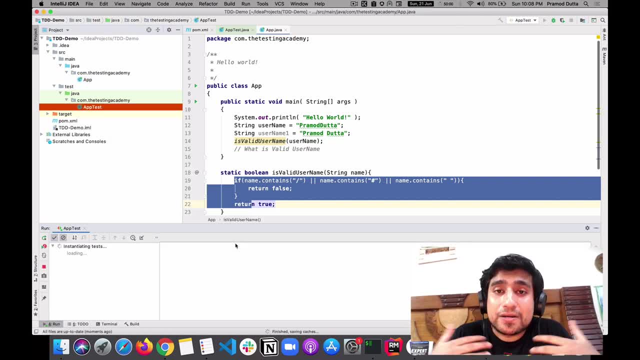 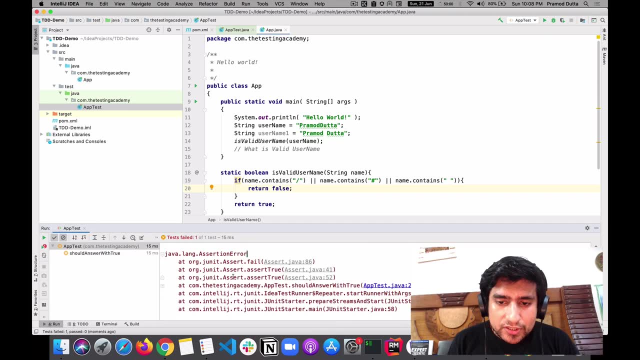 you can run your test cases. if all of test cases you are passing, it means it's completed, right? so, as you can see, it is failing. uh, so let's see how, why it is failing for it and which one for it. so let's see. yeah, username one. 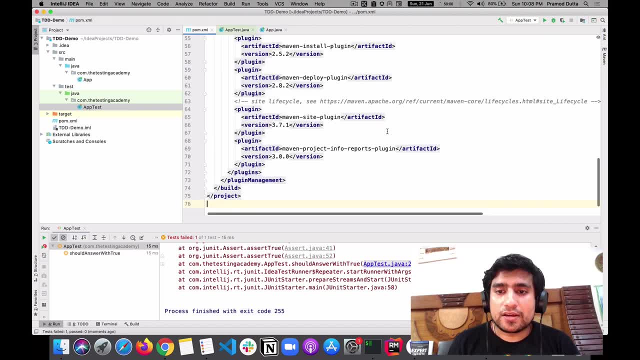 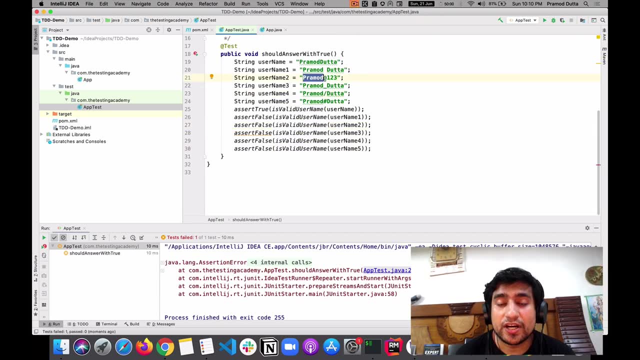 it is failing because space is not allowed, right, and here we have checked for it, right, it will return false in that case, right? so, uh, we need. what we are doing here is that, uh, we are writing the functionality right. so, for, at the rate it was failing, i have written name dot contain: 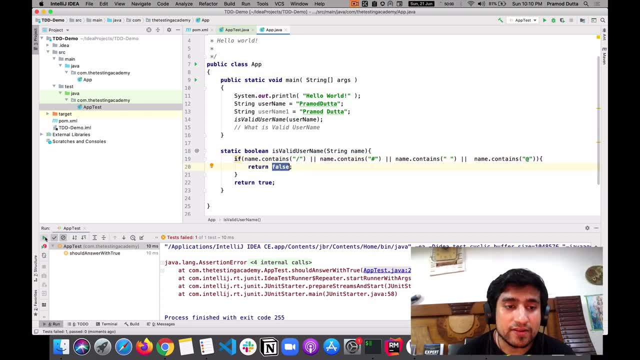 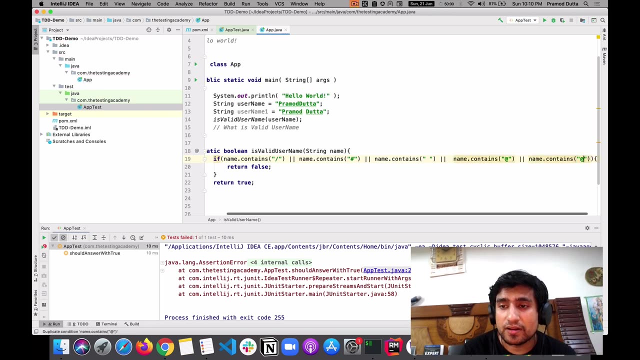 should be, it will be. if it should be a false one. now again, if i run it right, it will fail for this one because it will say that username 3 is underscore, right? uh, so let's add the underscore also. so now, with the test case, i'm writing the code if you can see right. so underscore, if it. 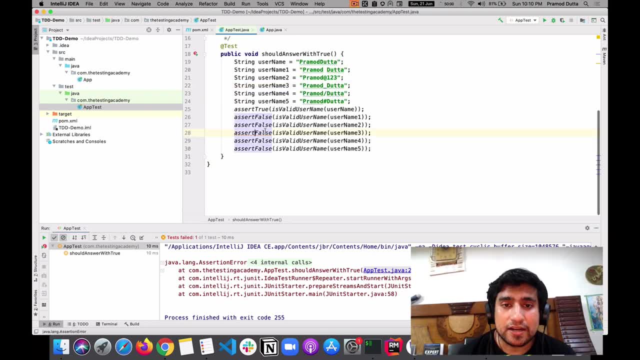 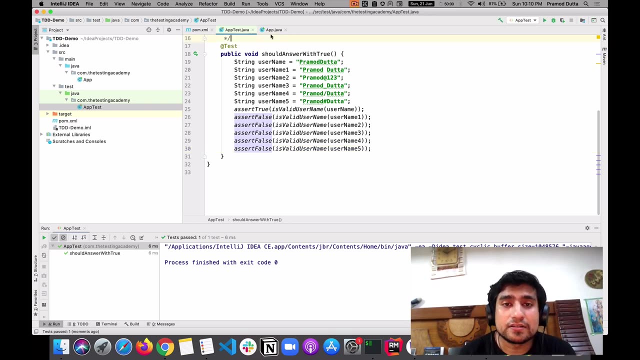 contains. i want to return false, right, and these are the false test cases. so i'm just resulting the false in that case. so, oh, yeah, let's run it again. so all the test cases are passed. it means that our functionality is now complete, right, and this is the function that we wanted to use. so this is like a test driven development process. 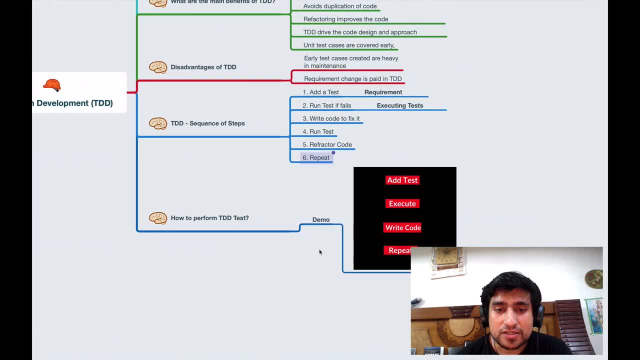 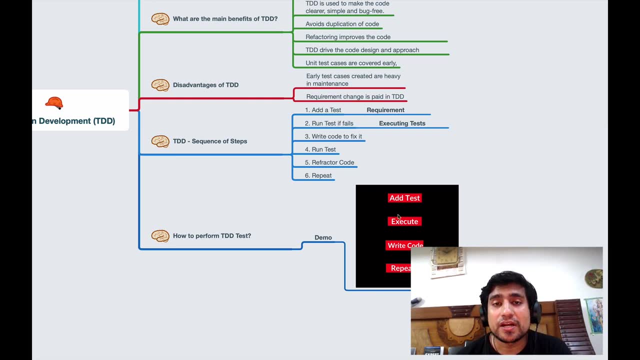 right. i hope you are able to grasp it. it's a very simpler process, uh, and where you just add the test case first, execute it whatever it is failing, you write the code and you just repeat it right, and you refactor the code again and again. right? thanks a lot for watching, i hope.